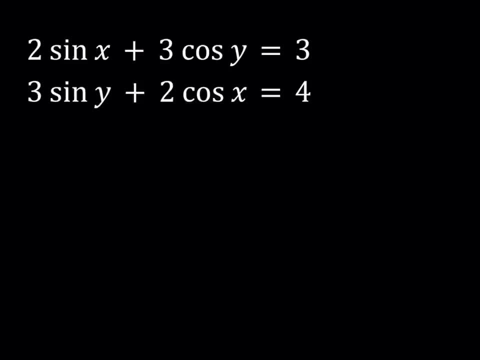 equal to 4. And we're going to be looking for x and y values. Now, there's a lot of different things you can do with systems, but especially for trigonometric systems, we have different options because of the identities that occur. One of the most important identities in trigonometry- 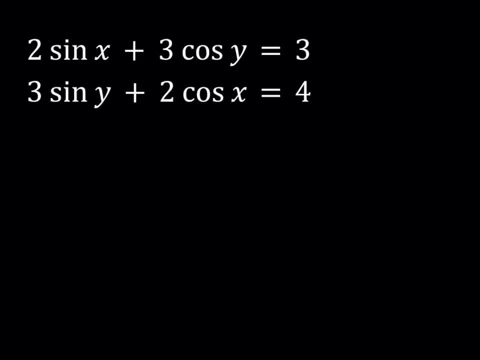 in my opinion, is the Pythagorean identity, which goes as: sine squared alpha plus cosine squared alpha is equal to 1.. Now, this is very important and you can easily prove it, you know, using a right triangle or by other means. but let's go ahead and use this to our 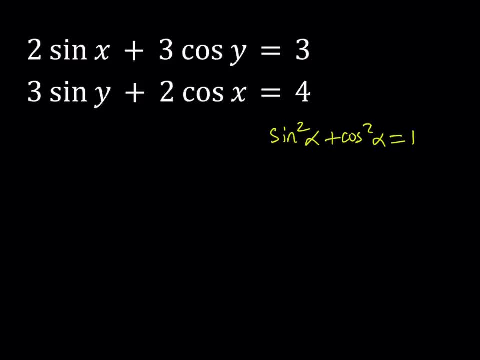 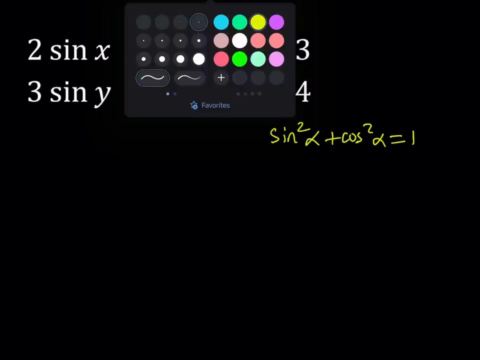 advantage Now for this purpose, since I do see that, for example, I have here 2 sine x and 2 cosine x- they have the same coefficients, and sine y and cosine y have the same coefficients. To take advantage of the Pythagorean identity, I would like to go ahead. 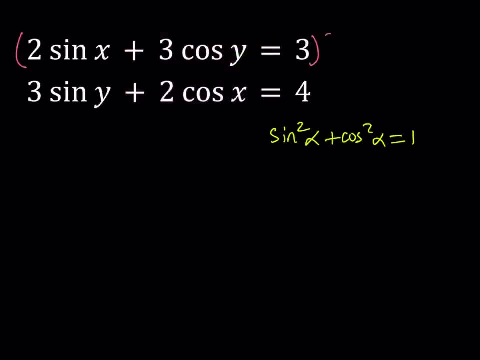 and square both sides of each equation and then see what happens from there. Okay, so once I square the first one, I should be getting something like 4 sine squared x plus 12 sine x. cosine y is equal to whoops. we forgot the last term, which is 9 cosine squared y, and that should. 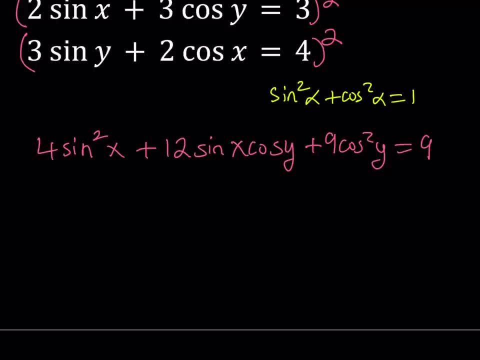 equal 9.. And if you square the second one, that should give you 9 sine squared y plus 12 sine y cosine x right plus 4 cosine squared x, and that should equal 4 squared, which is 16.. Now 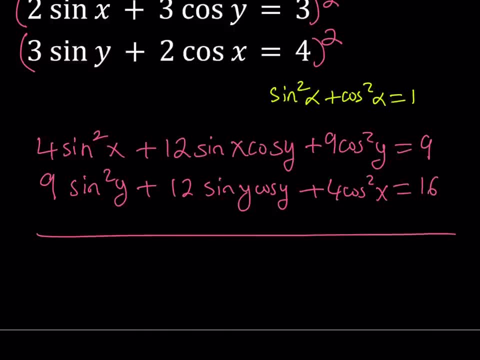 what I'd like to do is: I'd like to do this, I'd like to do this, I'd like to do this. I'd like to add these two equations, because notice that we have 4 sine squared here and 4 cosine squared. 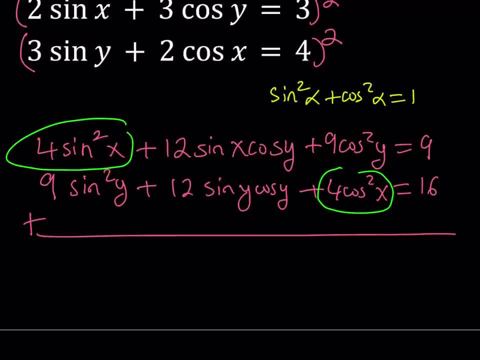 here, And obviously this means 4 times the quantity sine squared x plus cosine squared x, which is equal to 1, so that should give us a 4 there, right? So 4 times y is equal to 4.. We have 9 sine squared y and 9 cosine squared y. their sum is going to be 9, for the same reason. 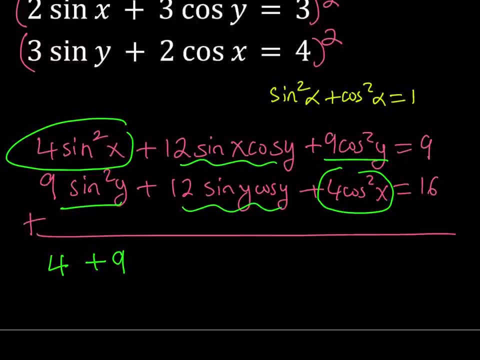 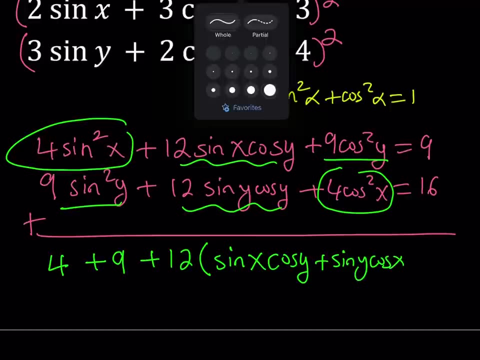 And then these two terms basically have the same coefficients, so I can just go ahead and factor and see what happens from there: Sine x- cosine y plus sine y- cosine x. By the way, this should be a cosine x, not a cosine y. Okay, so let's go ahead and fix that. This should be a cosine x, Okay. 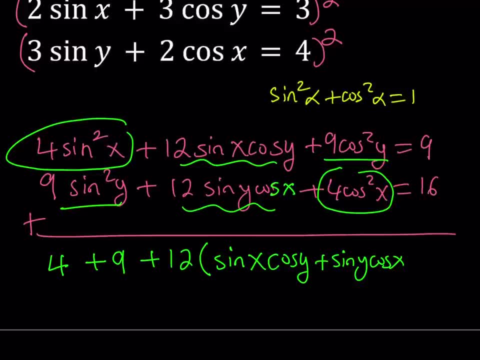 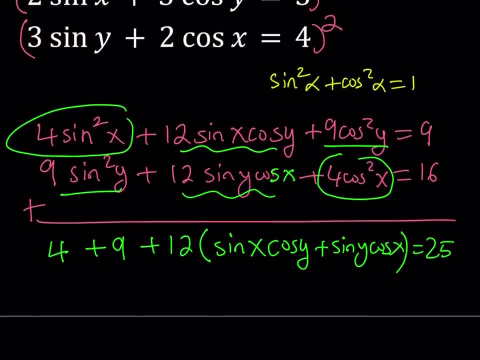 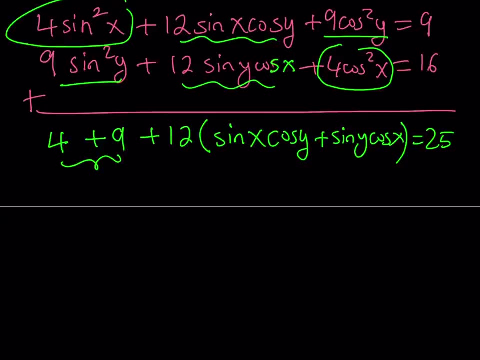 All right, so, and that should give me a sine y, cosine x. And then, on the right-hand side, I do have 9 plus 16, which is equal to 25.. Okay, So 4 plus 9 is equal to 13.. If I subtract 13 from 25, I get 12.. So I'm basically getting 12 times. 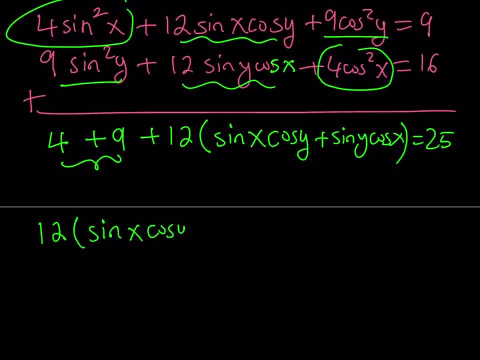 this quantity: sine x cosine y- and I'll tell you what it is in a little bit- plus sine y cosine x, is equal to 12.. Great, So we can divide both sides by 12, and we end up with a simpler expression. 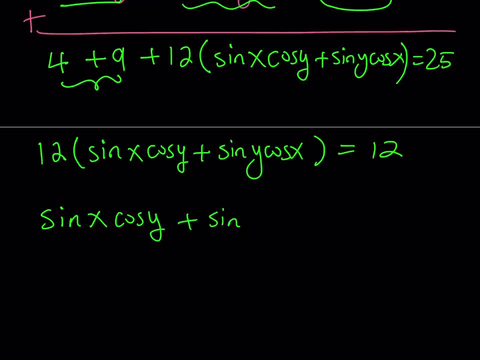 But now, what is that expression equivalent to? Now, you need to know the trigonometric identities, and there's a lot of them. But of course, there are some trigonometric identities, and there's a lot of them. But there are some patterns that you can take advantage of. For example, this one is the sine of. 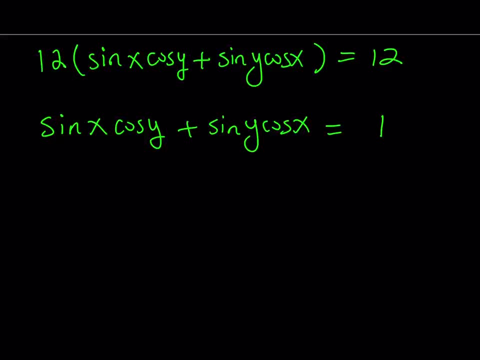 x plus y. It's a sum formula that you do definitely need to know And if you didn't now, hopefully you know when you start memorizing. Sine of x plus y is equal to that. So that's significant because we're basically taking a sum of products and then turning it into something simple, especially like 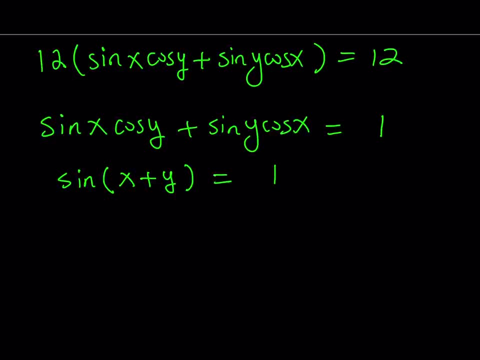 single sine. So that's really nice, Very compact, right? So this gives us sine of x plus y is equal to 1.. Now what is that supposed to mean? So let's go ahead and use our unit circle here. So what does? 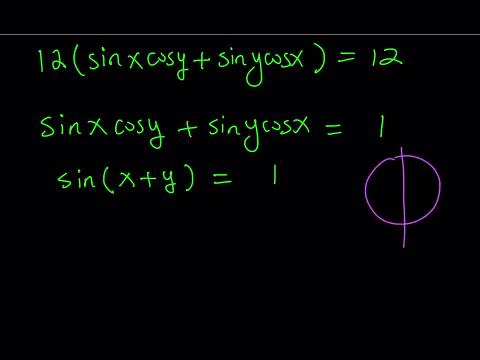 it mean for the sine of an angle to be 1?? Well, that doesn't always happen, right? That's kind of rare. Well, if you think about the unit circle, a circle whose radius is 1 and center at 0, 0,. 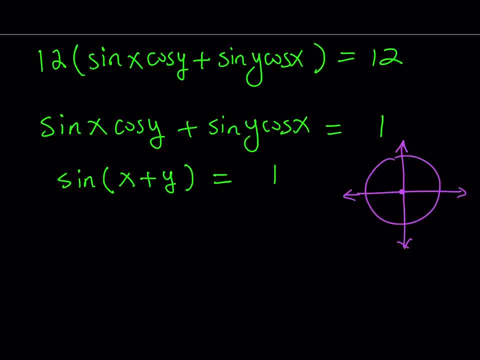 which is the origin. you're basically talking about the following. So I'd like to make, I'd like to make a right triangle here, But any right triangle that I make will have a hypotenuse of 1 because of the radius of the circle. So when, since we define sine of an angle as opposite over. 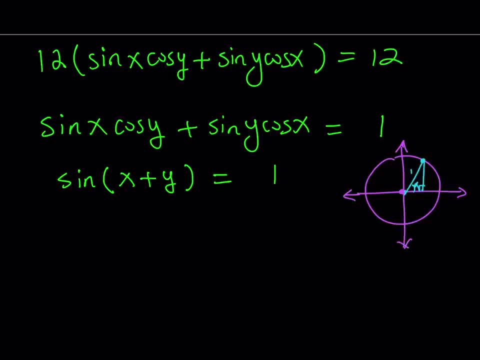 hypotenuse. when the hypotenuse is 1, the sine of the angle is just going to be the opposite side length, or the coordinates for this purpose, And it's just going to be the y coordinate in this case. In other words, what I'm trying to say is, on the unit circle, the angle whose sine. 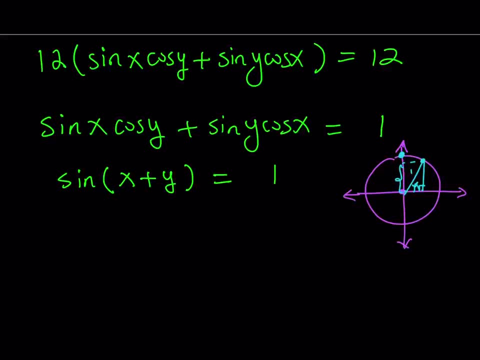 is 1, is pi over 2 in terms of radians, right, But we can also write it this way: Well, x plus y is not just pi over 2, because we can also definitely add multiples of 2 pi. So let's just go ahead and. 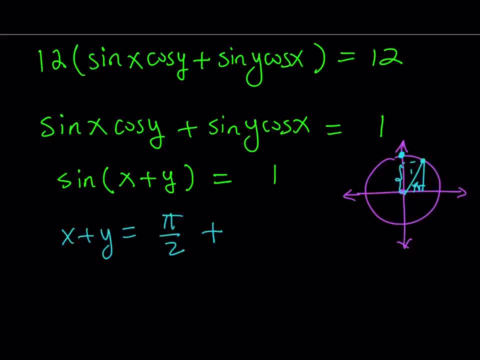 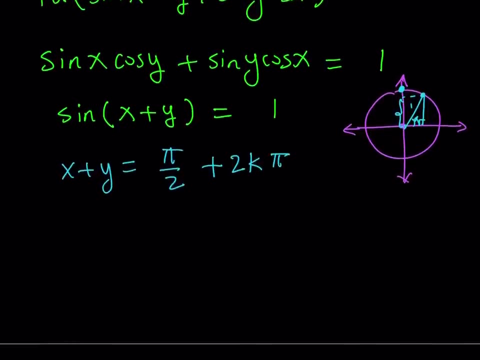 you know, just add 2 pi, multiply by k. So let's just write it as 2k pi. All right, I want to express it in a nicer way. So let's go ahead and do the following. I can just write it as making. 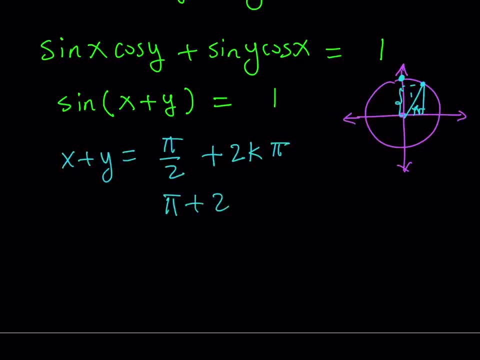 a common denominator. I can make it pi plus 2k, 2k pi, And I'm going to multiply that by 2.. Of course, that's going to be 4k pi divided by 2, like this. And what I'd like to do is I'd like to factor out a pi here so that 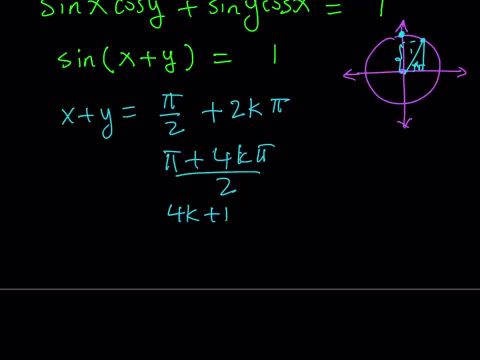 when I do, I get 4k plus 1.. And I'd like to multiply that by pi over 2.. So basically we're talking about multiples of pi over 2 here, and not just any multiple of pi over 2, but odd multiples. 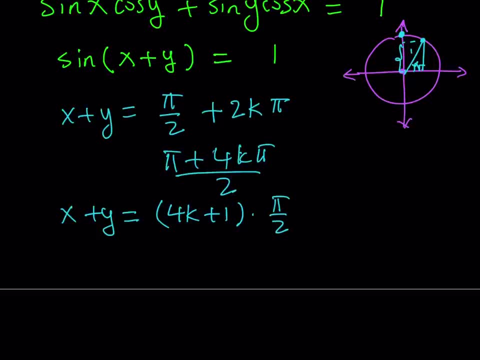 of pi over 2, but not all the odd multiples We're kind of skipping. So 4k plus 1 is kind of like a numbers that leave a remainder of 1 when divided by 4, numbers like 1 or 9 or 13 and so on and so forth. So we're only hitting this positive. 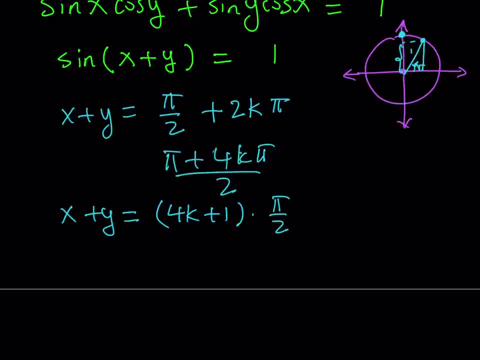 value, because if you just say odd multiples of pi over 2,, then you're also talking about 3 pi over 2, which is a negative value. Okay, So those are my x plus y values. Now, this is important because if x plus y is, for example, pi over 2,, then you can safely say that. 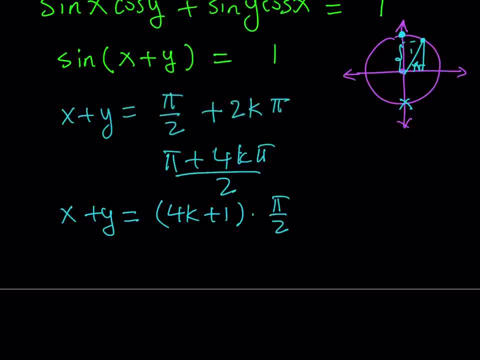 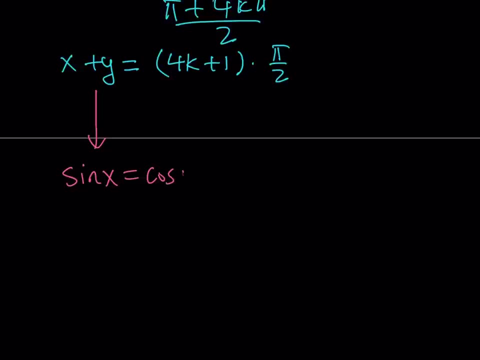 sine and cosine of x and y are related. What is that supposed to mean? It just means that sine x is equal to cosine y, because you're basically talking about two angles that are complementary And if you draw a right triangle and you know, label two angles that are. 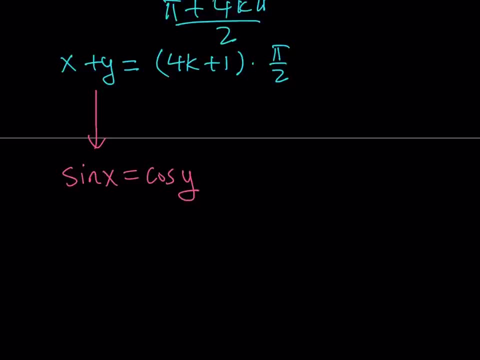 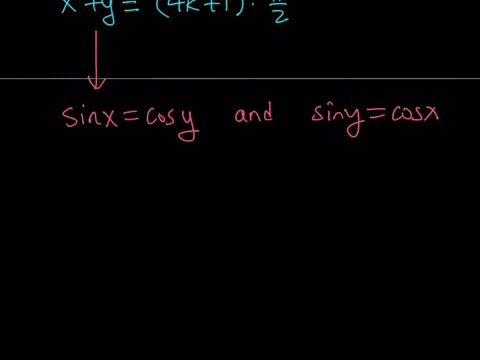 complementary, you'll notice that sine of x is going to be the same as cosine of y And, of course, it's also true that sine of y is equal to cosine of x. We're going to use the original equations now. Okay, Our original equations were 2 sine x plus. 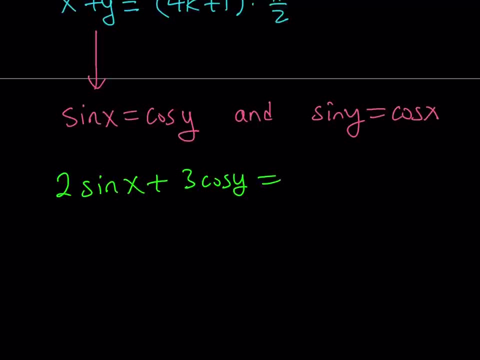 3, cosine y is equal to 3.. Now in this equation, if you go ahead and replace sine x with cosine y, you get 5: cosine y is equal to 3.. And that gives you cosine y is equal to 3, fifths Now: 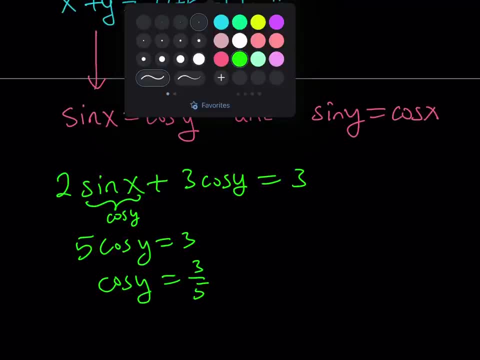 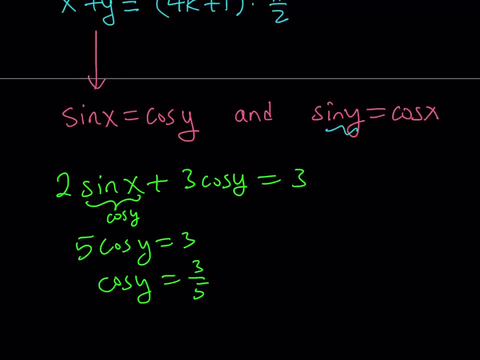 if you do something similar, if you do something similar for the other one, for example, replace sine y with cosine x, right here. And what was our original equation? Of course we have to go to that first. So that was 3 sine y. So that was. 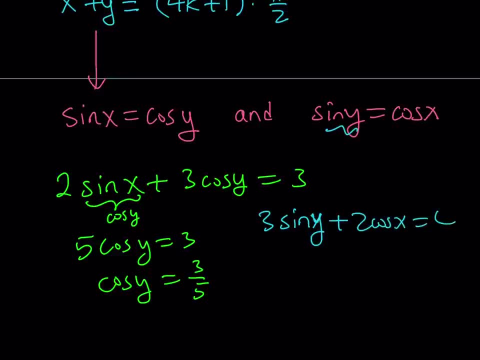 3 sine y plus 2 cosine x is equal to 4, right, So let me go ahead and, you know, fix this so it looks nicer. So in this equation we can basically replace sine y with cosine x, So we get 5 cosine. 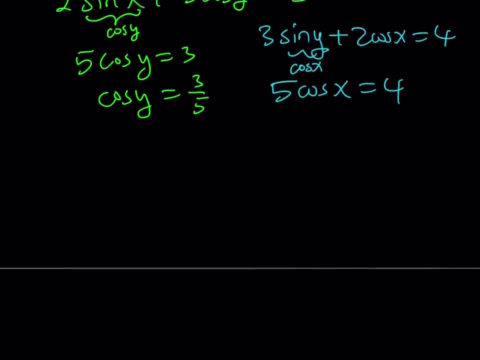 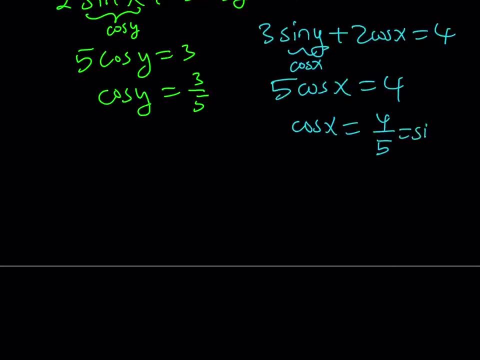 x is equal to 4.. And that just means that cosine x is equal to 4 fifths. So we got like 2 different values here. Of course, cosine x is the same as sine y And cosine y is the same as sine x. So all these- 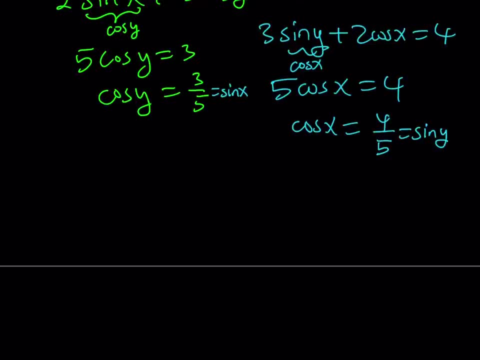 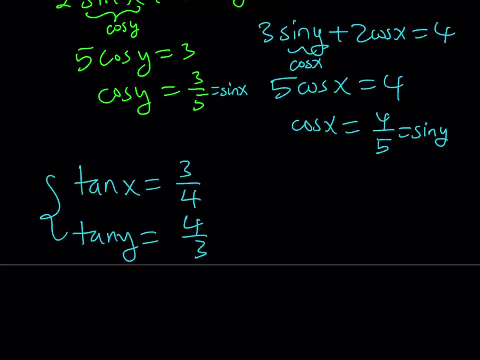 values are obviously positive. So we can safely say that from here tangent x is going to be 3 fourths And tangent y is going to be 4 thirds. So basically you're talking about 2 angles here whose tangents are reciprocals. Of course these angles are complementary, Let's remember. 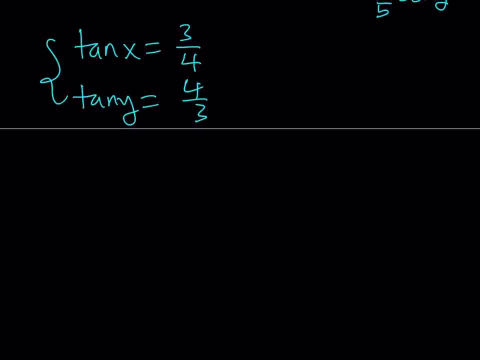 that, So we can write our result as follows: So from here x becomes tan inverse of 3 fourths, And of course we can add multiples of 2 pi. So let's just go ahead and add 2 n pi to it. 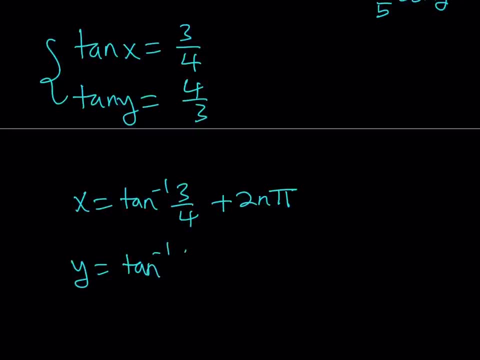 And then y can be written as tan inverse of 4 thirds, And then we can again multiply or add multiples of 2 pi to it. Let's just write it as 2 l pi, where n and l are integers. So for some integers n and l. 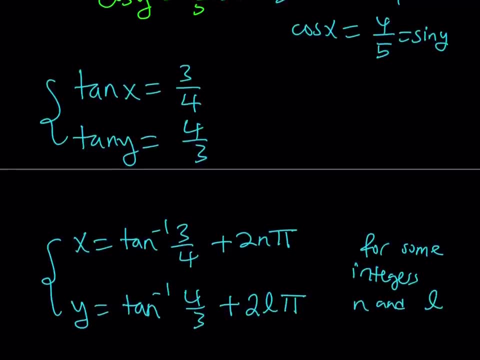 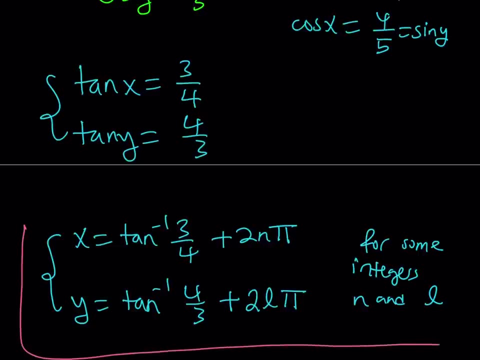 this is going to be true And that's basically going to give us all the solutions to this system. Well, this brings us to the end of this video. I hope you enjoyed it. Please let me know. Don't forget to like, comment and subscribe. I'll see you tomorrow with another video. Until then, 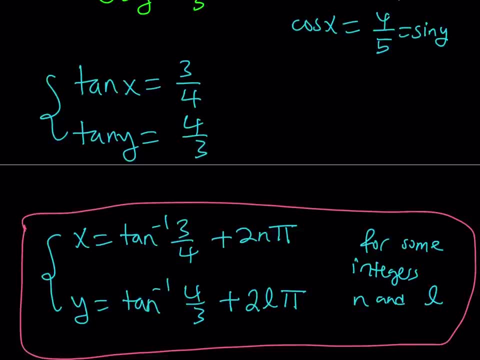 be safe, take care and Bye-bye. 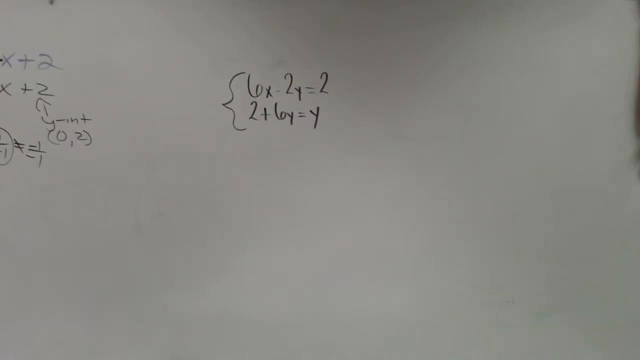 So in this example, ladies and gentlemen, what we have is: 6x minus 2y is equal to 2, and 2 plus 6y equals 2.. So, basically, what we're doing for this is: I'm asking you just to graph each one of these separately. 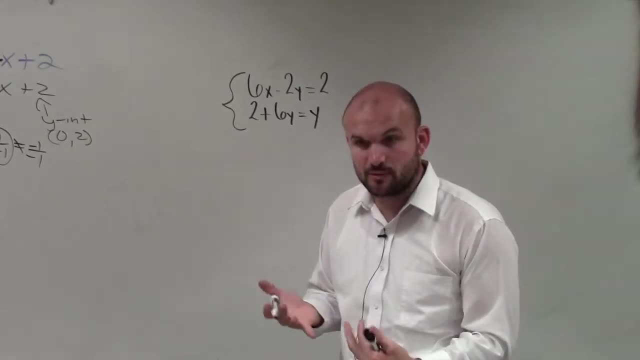 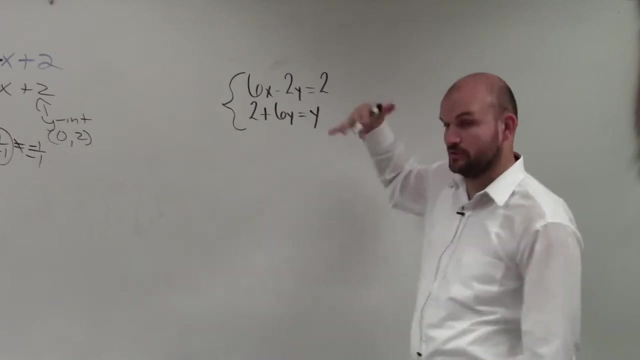 and identify where they intersect, So to graph them. basically, what I'm going to do is there's two different ways we can graph: We can use intercept method or we can use slope-intercept method. I think the easiest thing for me to be able to do is rewrite these in slope-intercept form. 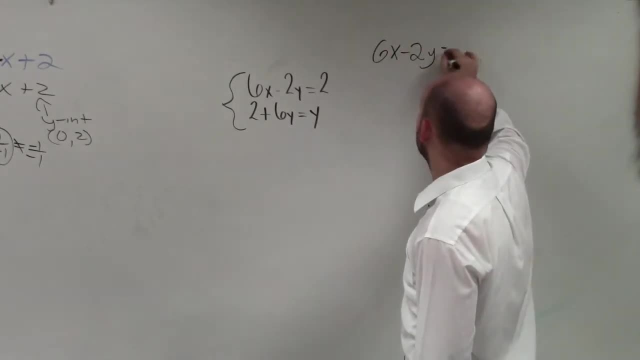 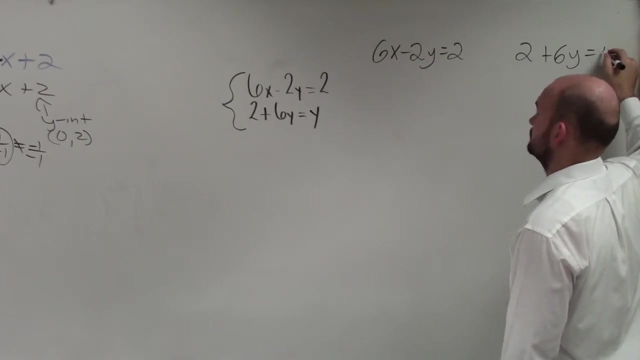 So I'll take write both equations and I will rewrite in slope-intercept form. Oh, that's 6x. Hey, Jason, that's not what you need to be doing right now. So now, for each one of these, I need to solve for y. 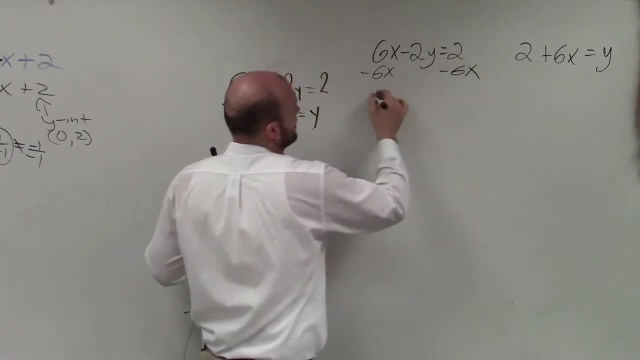 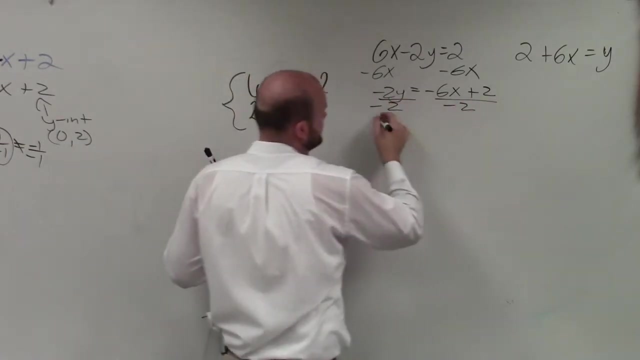 So I'll subtract to 6x. subtract to 6x, I have negative 2y equals negative 6x plus 2.. Divide by negative 2, divide by negative 2. y is equal to a positive 3x minus 1.. 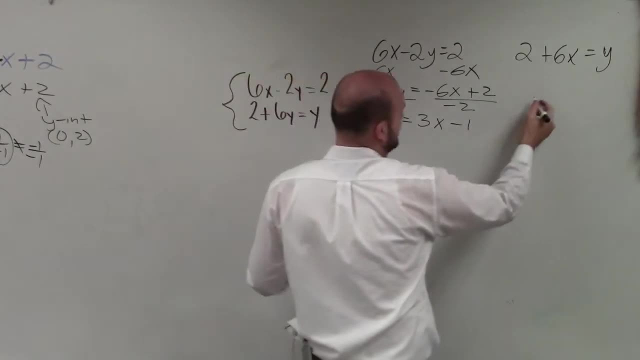 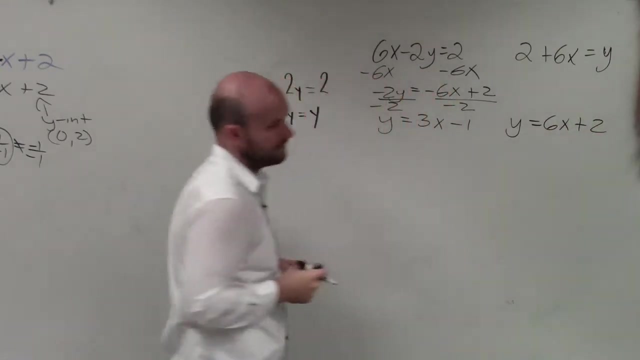 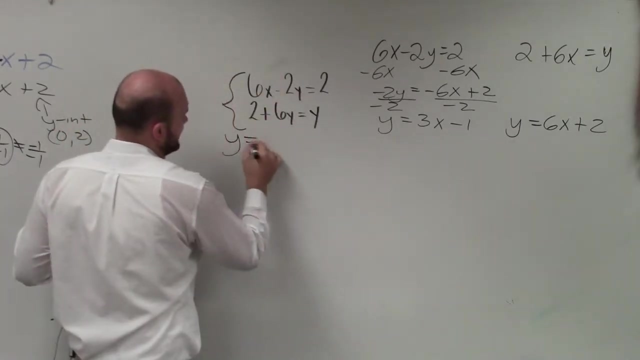 Is everybody fine with that? This one is already solved for y, so I'm just going to rewrite it as y equals 6x plus 2.. Okay, So now I've solved them both in slope-intercept form. Now it's very important when we have slope-intercept form, which is our: y equals mx plus b. 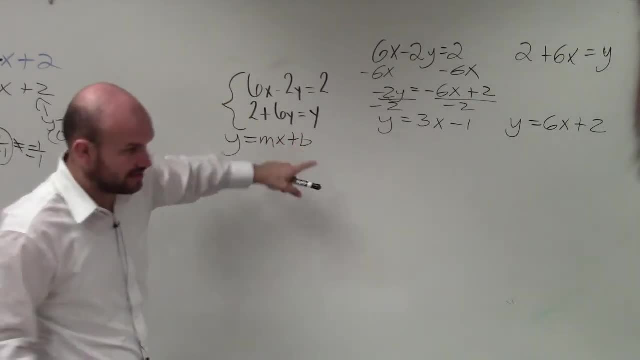 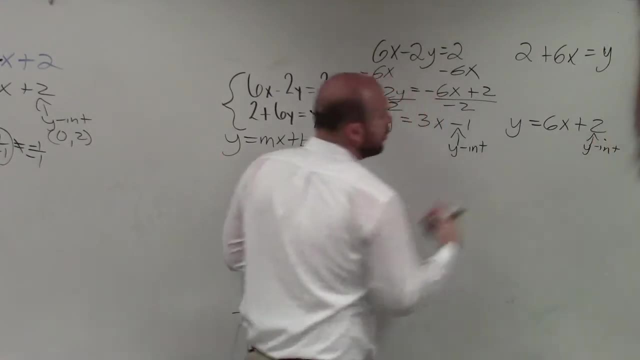 for us to understand what does. What does m represent? What does b represent? Remember b represents your y-intercept And remember y-intercept is a coordinate point. 0, negative 1.. 0, negative 1..